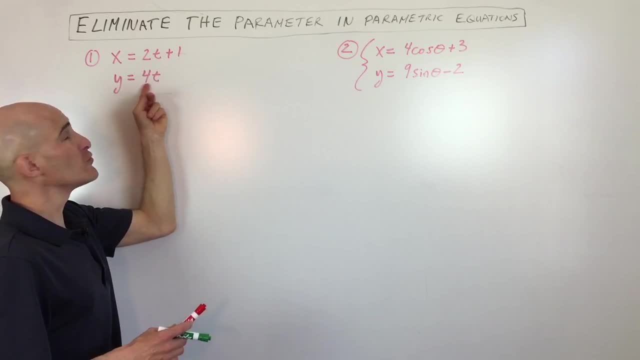 Parametric equations are usually composed of, you know, two parts and you can see this is like the horizontal component, the x component as a function of t- Usually we think of t as time- and then over here we have y, which is like the vertical component, and then that y value is a. 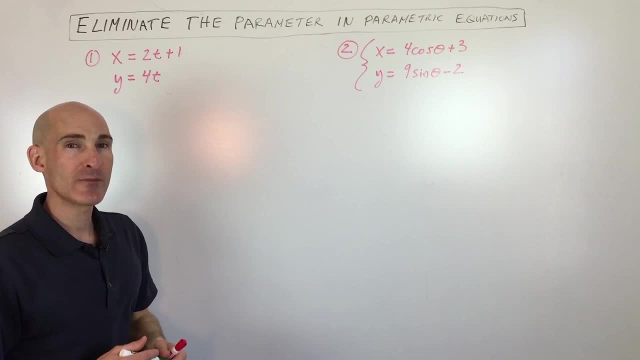 function of time as well. But what we want to do is we want to eliminate that parameter t and just get an equation in terms of x and y. So let's see if we can do that. So in this example, what we're going to do is we're going to solve for t in that top equation. So we're going to do that. 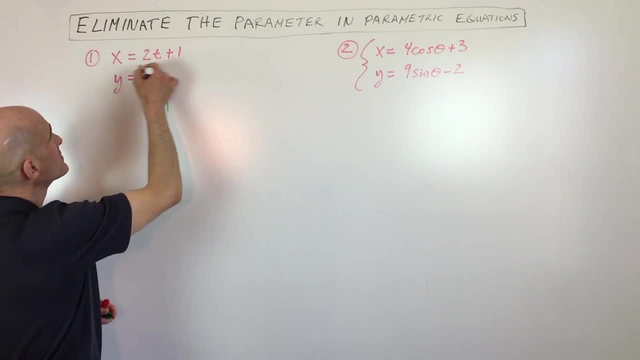 by getting t by itself. So x minus 1 subtract the 1 equals 2t. We're going to divide by 2, okay, so that now we have t equals x minus 1 over 2.. Now if we put that in for t in the second equation, 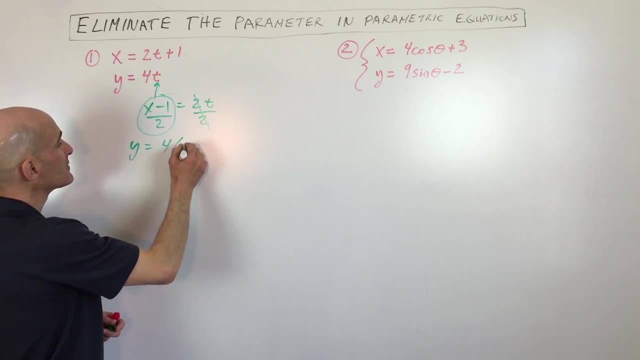 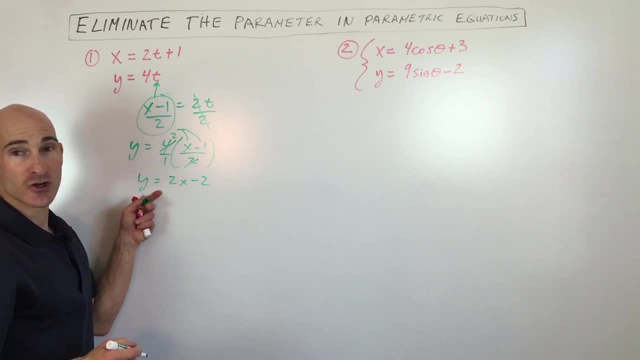 x minus 2.. So now we have an equation just in terms of x's and y's. If we want to graph it, what you can do is, of course, we can graph this just as a slope intercept form of a line, The. 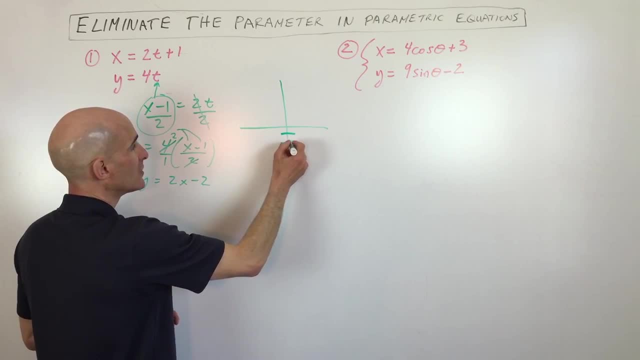 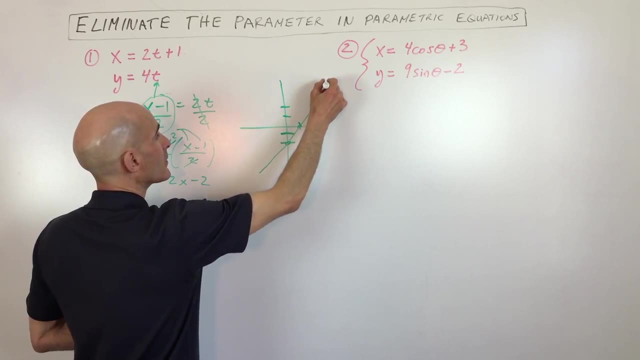 slope is going to be 2 and the y intercept is negative 2.. So we're going up 2 over 1, up 2 over 1.. And there's our line right there. But the other component of this that you want, 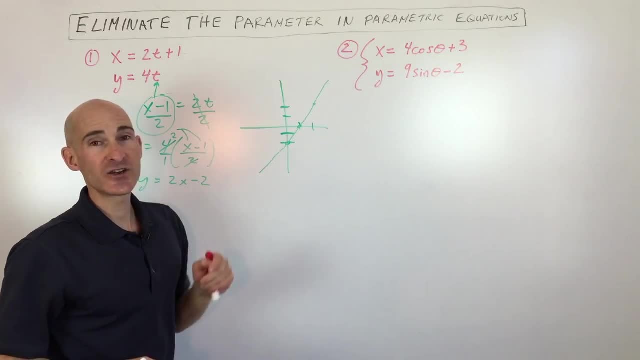 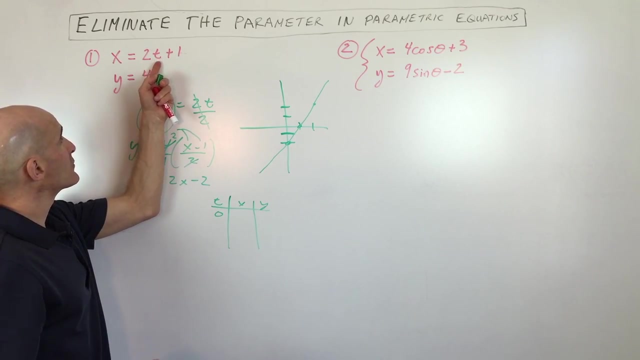 to pay attention to is the direction. So are we going this way as t increases, or are we going this way as t increases And what you can do is just make a quick table, okay, like this, And you can just say: all right, when t is 0, what are the x and y coordinates? So if I put 0 in for t here? 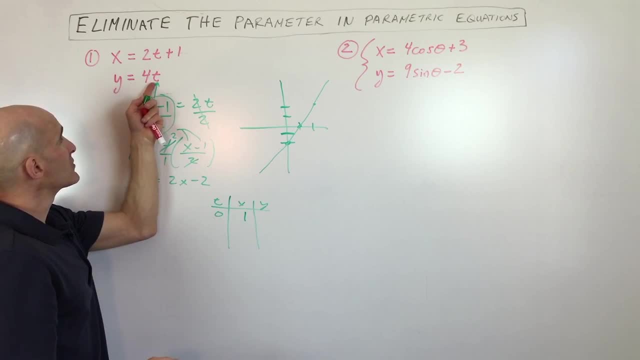 you can see I'm getting x equals 1.. And if I put 0 in for t here, you can see I'm getting 0, okay, And then if I put t equals 1, that's 2 plus 1, which is 3.. And if I put 1 here? 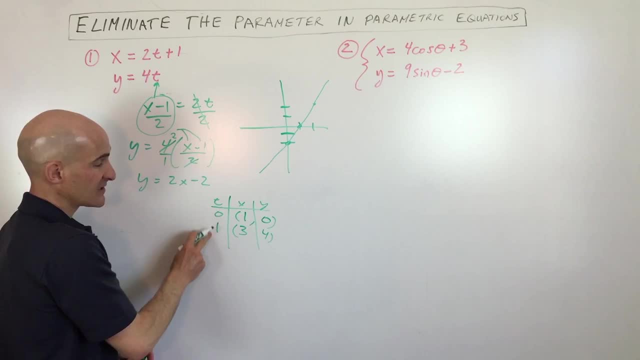 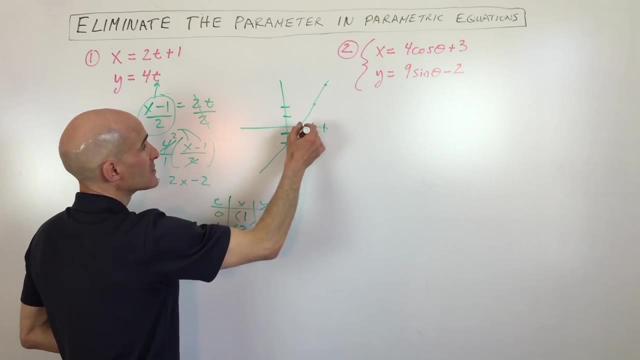 I'm getting 4.. So you can see we're going as t is getting larger and larger, as it's increasing. we're going from 1, 0, okay- over to 3, 4.. So that means that we're going in this. 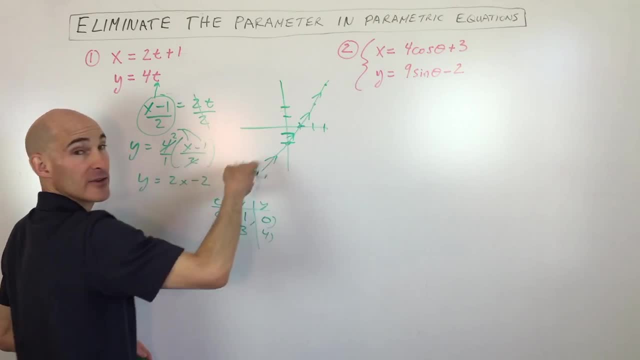 direction, And we can just indicate that with these little arrows along the line there. So with increasing values of t, we're going that direction along the line. Okay, now the second example. we're going to look at this one here. x equals 4 cosine theta plus 3, y equals 9 sine. 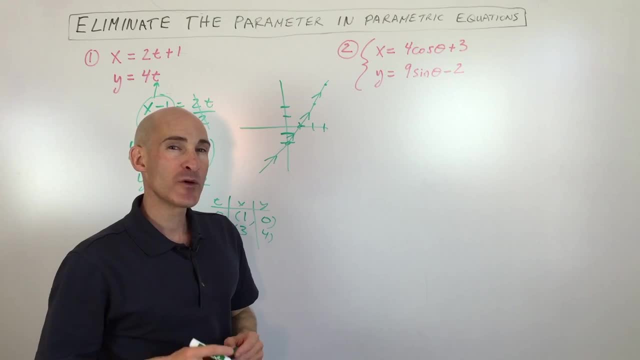 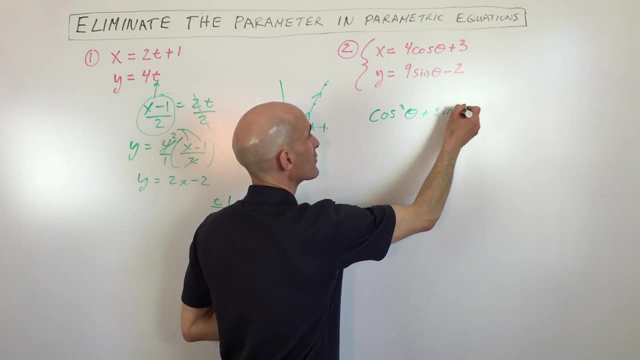 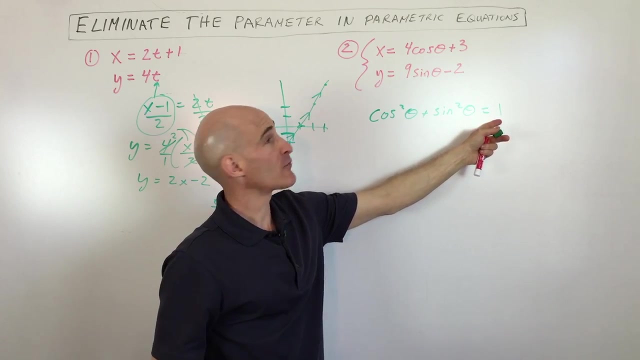 theta minus 2.. Now just a quick reminder. remember the Pythagorean trig identities. Remember this one here: Cosine squared theta plus sine squared theta equals 1.. Well, if you do, okay, we're going to use this. okay to again eliminate that parameter. In this case, our parameter is theta. 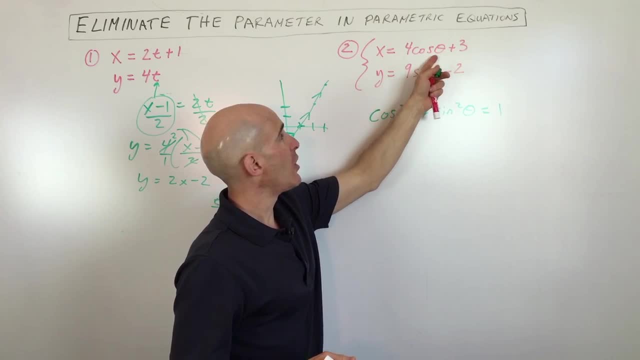 okay, the angle theta And the way we're going to do that is we're going to solve for cosine and we're going to solve for sine. So what I mean by that is we're going to get the cosine by itself. So in this top equation we're going to subtract 3 and divide by 4. So we get cosine- theta. 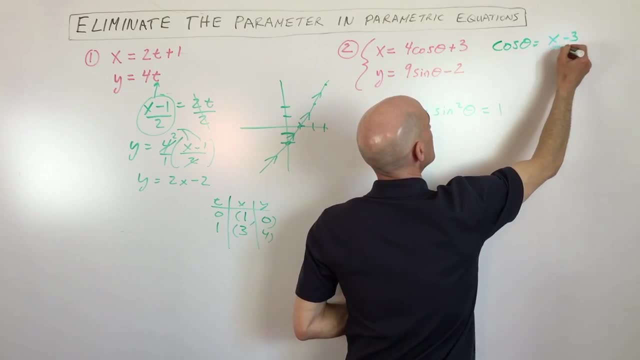 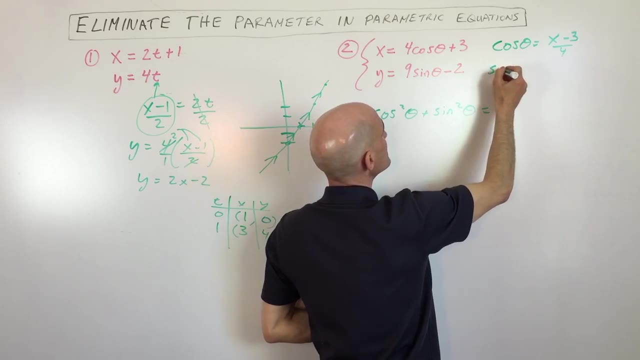 equals x minus 3, divided by 4.. Same thing in this bottom equation we're going to get the sine by itself. So we're going to add 2 and divide by 9.. So we get sine of theta equals y plus 2,. 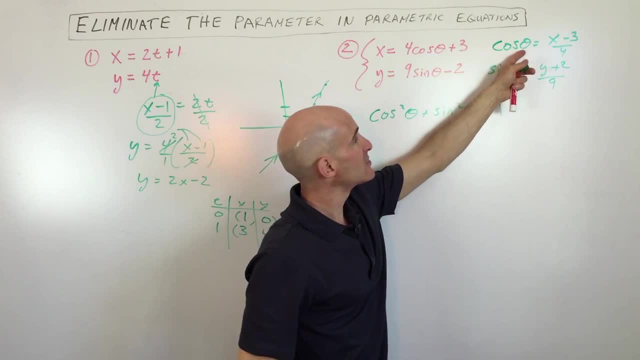 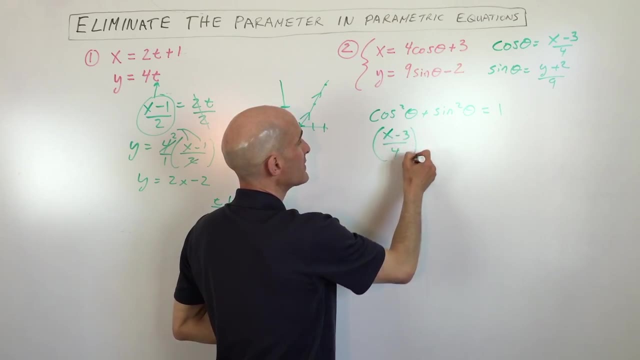 all divided by 9.. So now what we can do is we can substitute, in place of cosine, theta, x minus 3, divided by 4, the quantity squared, because you see, this is cosine squared plus y, y plus 4,. 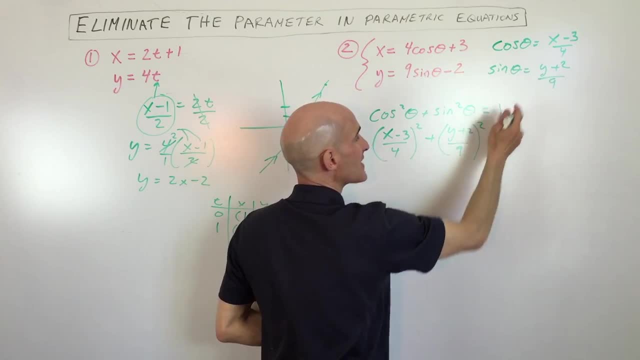 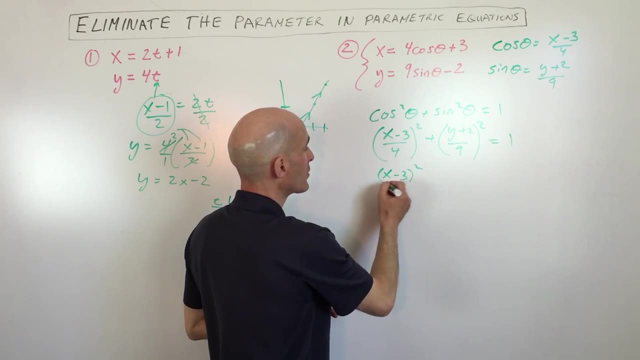 2 divided by 9 squared, since that's the sine of theta, and that equals 1. now, if we take it just one step further, simplify it a little bit more, we get x minus 3, squared over 16, plus y plus 2 squared over 9, squared of course, which 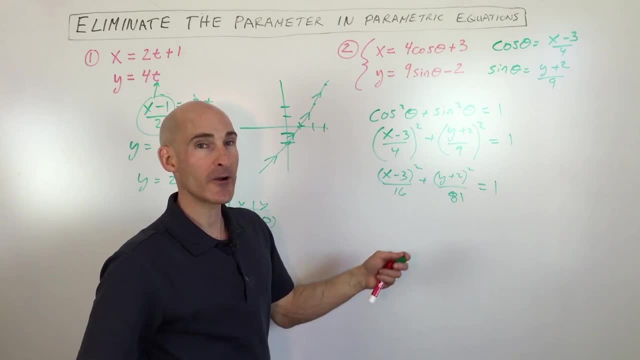 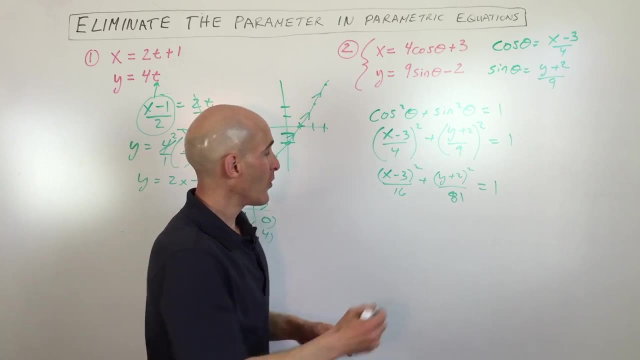 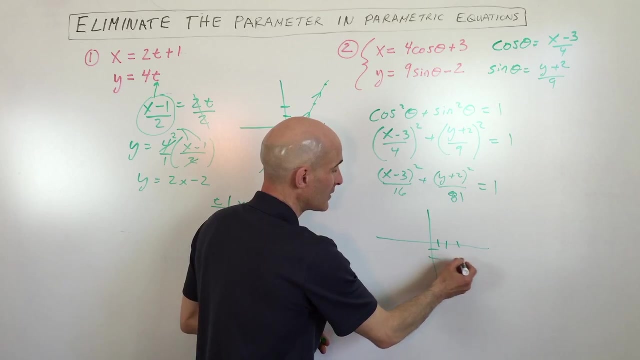 is 81 equals 1, in case they're with me so far. so this is the form of what type of a equation in ellipse, right? so if we want to graph this ellipse, you can see it centered at 3 negative 2. 1 2 3 negative 2. ok, we're going for the square. 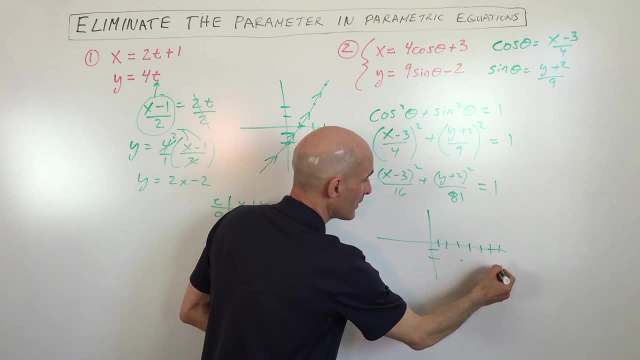 of 16. 4 in the x direction: 1, 2, 3, 4, ok, right there. 4 in the other direction: ok, and then the Y direction. we're going up 9 and down 9, the square root of 81. so that's 2, 3, 4, 5, 6, 7, 8, 9. right about there.